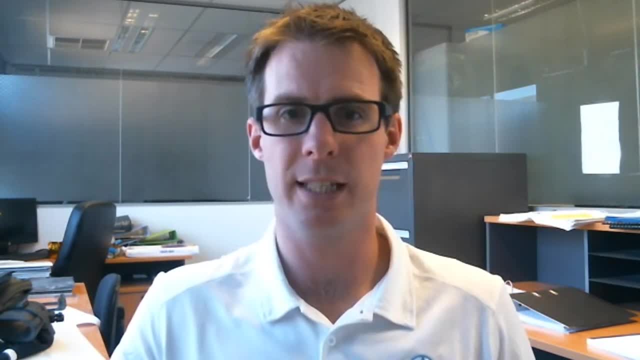 that are reading them. Secondly is to join us on LinkedIn, which is where we post most of our blogs in real time, so you'll get them as well. So just follow this link and click on LinkedIn and follow us there. That'd be great. 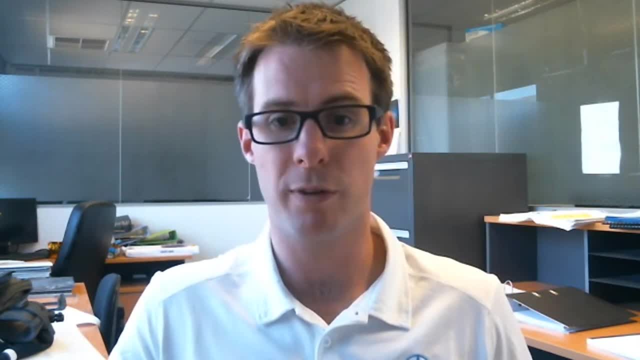 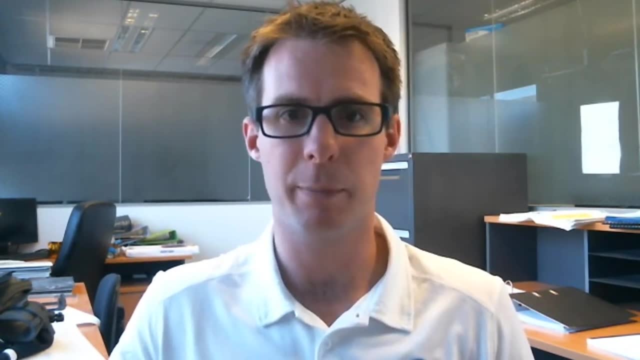 And then the third thing is to share it on your favorite social media platform. That'd be awesome. We'd really really appreciate that, so that more people can read the blog and find it and stuff like that. So that'd be cool. So let's just have a quick look at 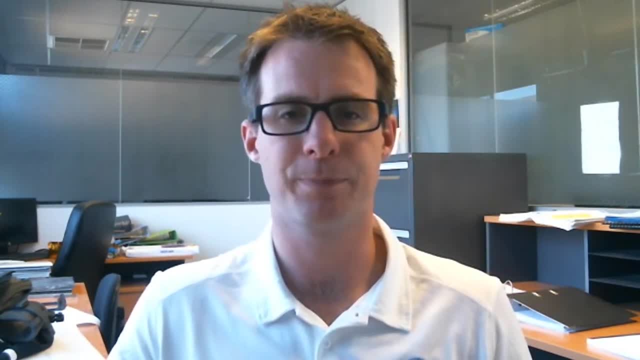 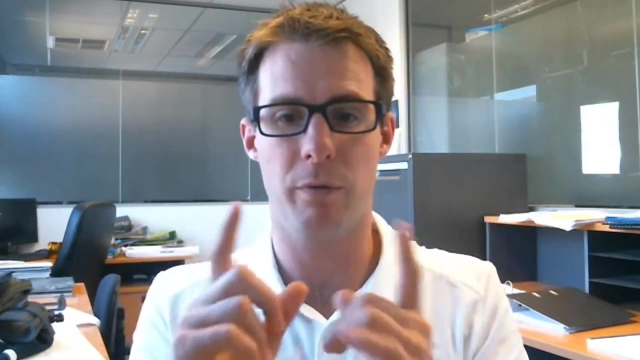 what is a contracts administrator in construction? So basically, in construction you'll have two parties to a contract. So one person wants something built, the other person is going to build it. Pretty simple, right? So between those two parties you'll have a contract and inside 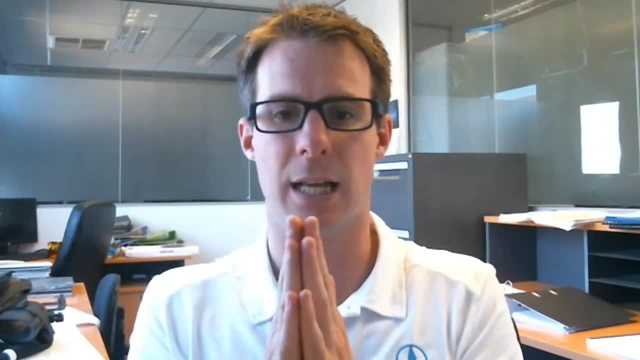 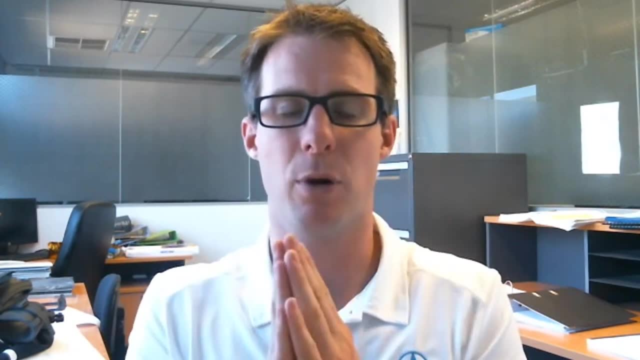 that contract you'll have a number of different clauses. that says you're going to be finished by this day. the job is going to cost this much. every month you have to submit a progress claim. to me Say, if the job is 12 months, that's, for instance, 12 progress claims which? 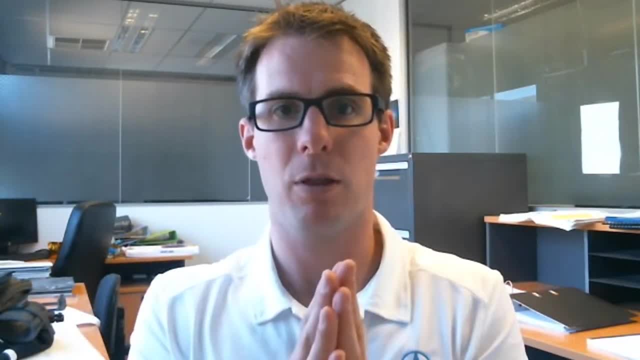 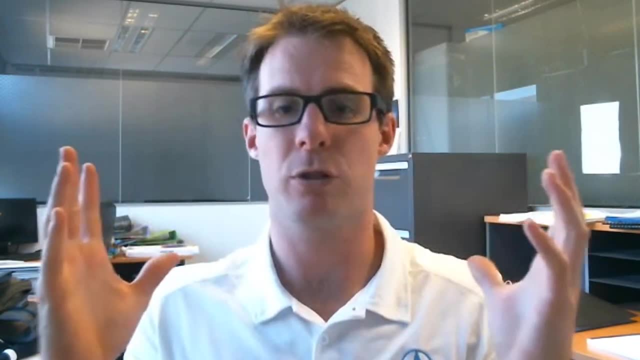 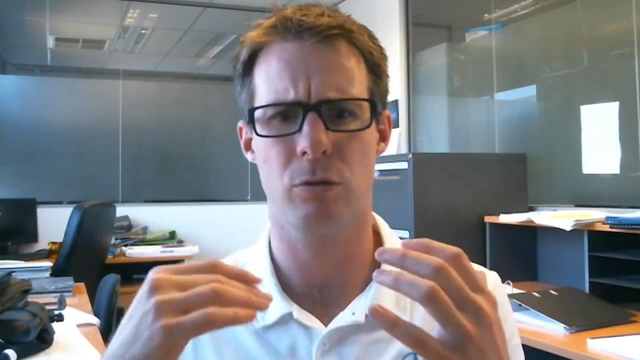 is basically how much money in that month have you actually work you've actually done, So basically you can get paid. And there's lots and lots and lots of other clauses. Some contracts are quite simple. some contracts are pretty complex and can sort of deal with a lot of different things. 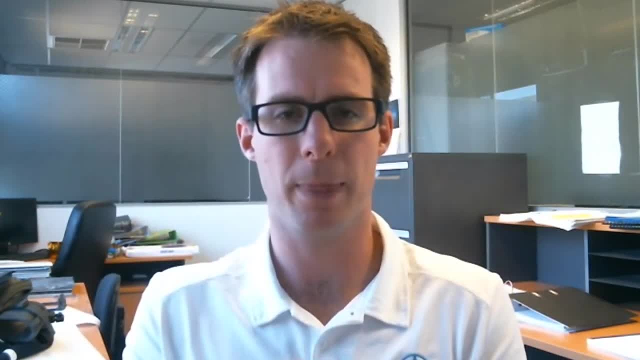 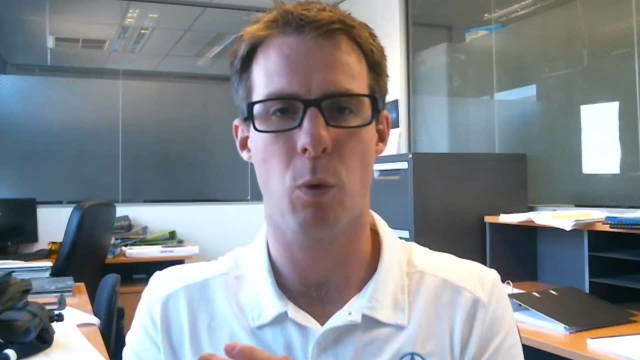 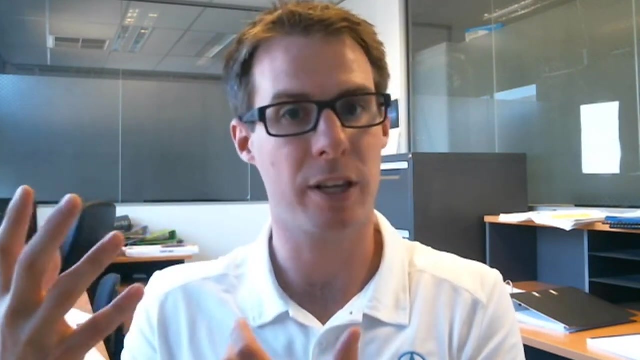 So, basically, what a contracts administrator is there to do is to go through the contract and find out all the different areas of deliverables that the contract requires. So, for instance, providing certain information at a certain time, Notifying of a contract, Notifying of certain things that happen at certain times. So, for instance, there was 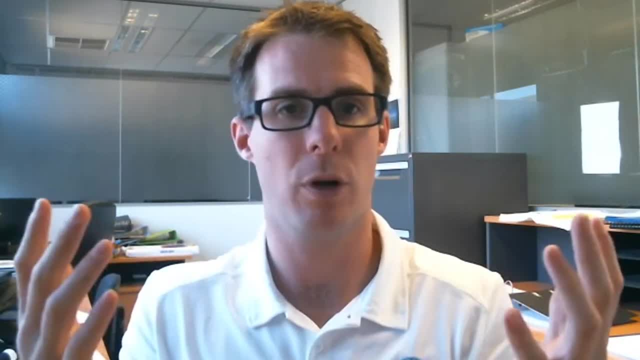 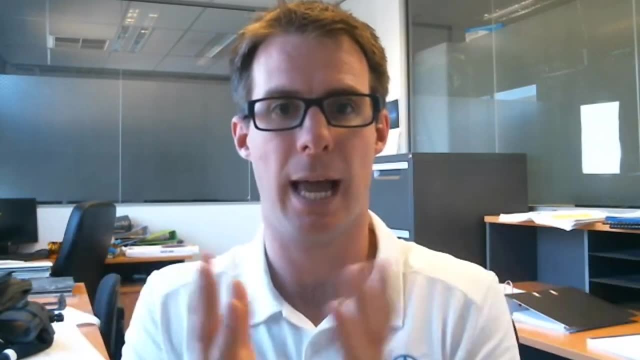 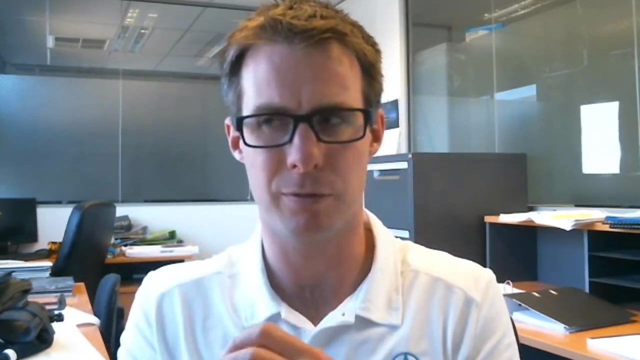 a delay in the works and the delay was a fault of somebody else, And basically notifying the other party that this has happened so that they can deal with that at the time. So a contracts administrator's job is very, very important in construction because legally,